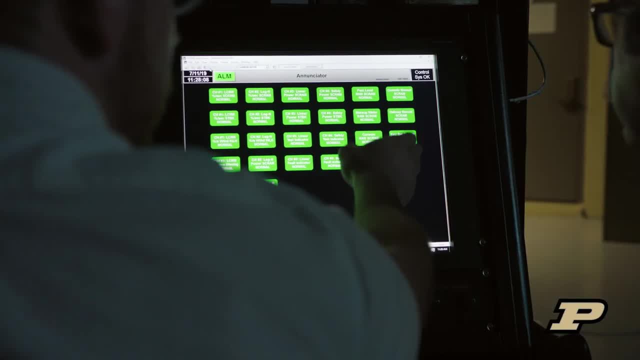 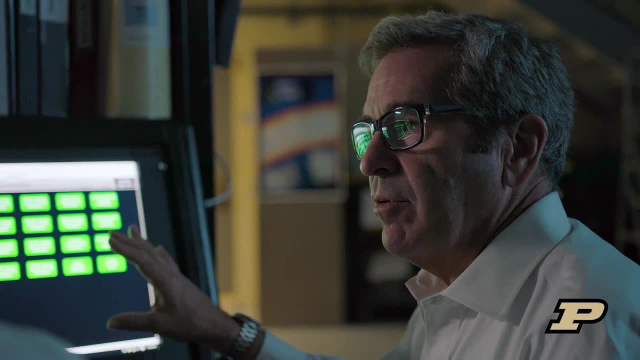 supervisor, Clive Townsend, showed me how the updated control panel gives operators much greater situational awareness. Is it more information than you could have gleaned from the analog system? It certainly is. I have an infinite number of screens that I could put in. I can have high. 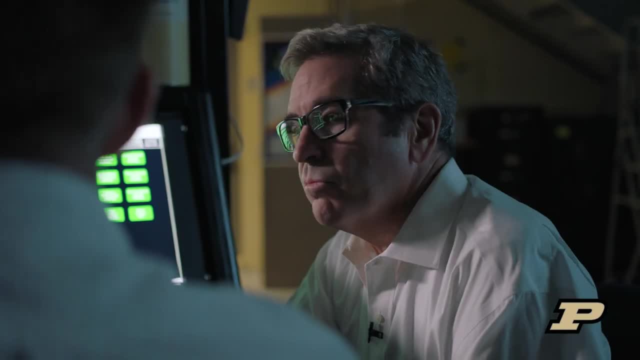 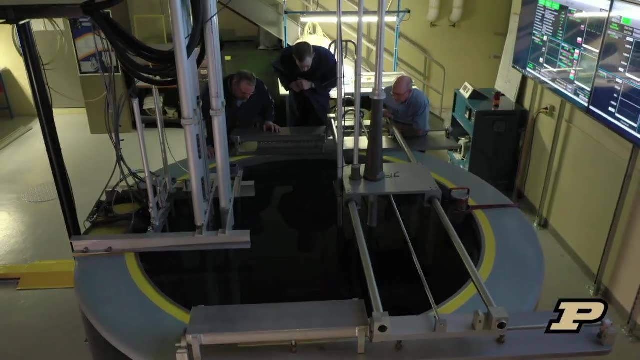 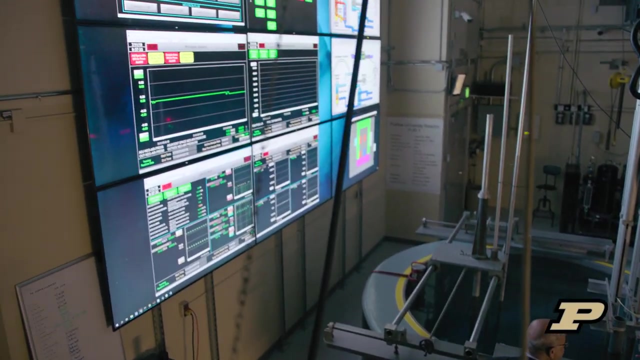 level information and then allow the operator to dial into that as necessary. We want to demonstrate that this system is reliable, safe and can do much better job than the analog systems. Almost a decade in the making, the 1.2 million dollar digitization of PIR-1 was funded by the. 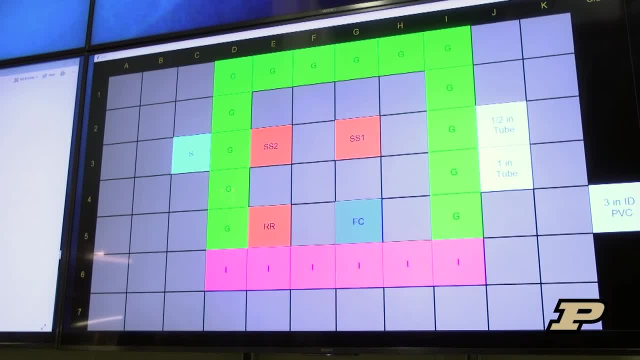 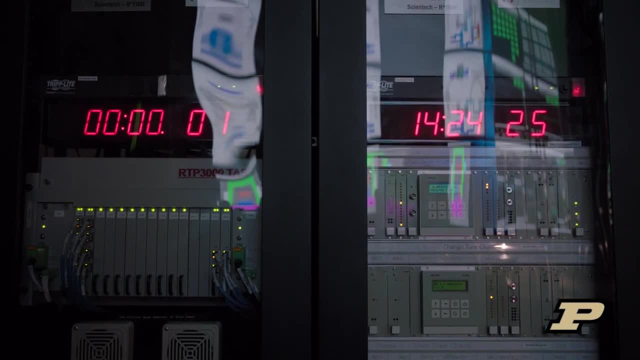 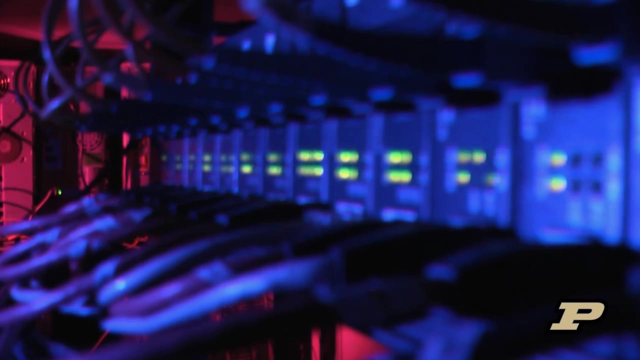 Department of Energy and the US Department of Energy And approved by the Nuclear Regulatory Commission. But bringing a nuclear reactor online in the virtual world carries its own set of risks. The threat of cyber mischief is on their minds here as well. We create new vulnerabilities. but we can create cyber physical protection systems to build. 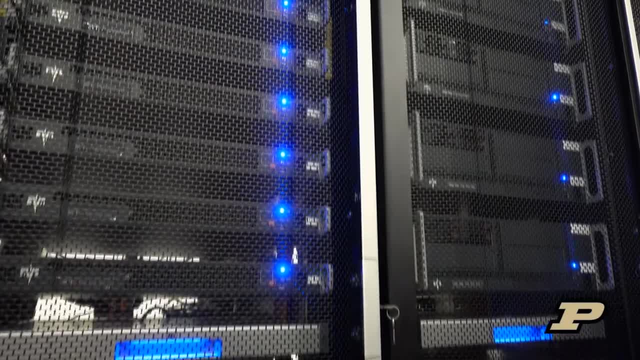 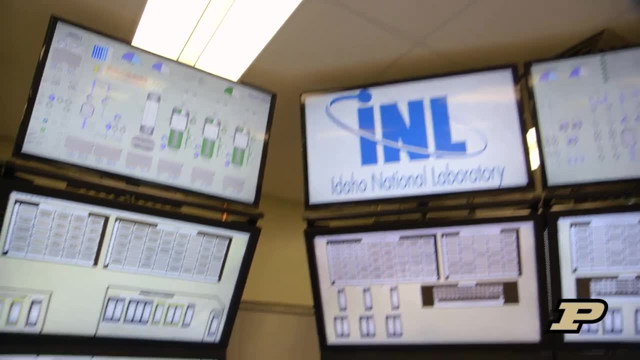 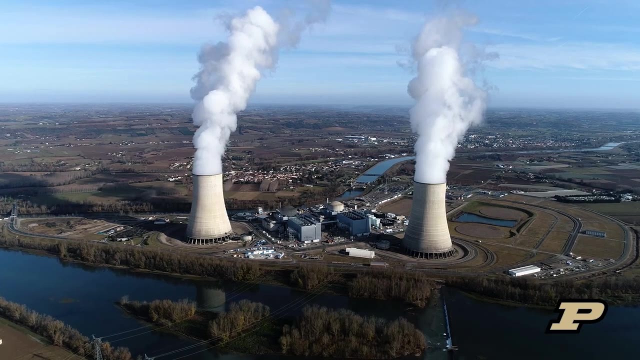 on the old safeguards and protect them in ways that are invulnerable to the dangers of connectivity MILES O'. They believe the pros outweigh the cons- That digital reactors, big data analysis and, ultimately, artificial intelligence will lead to safer, more efficient atomic power in the future. 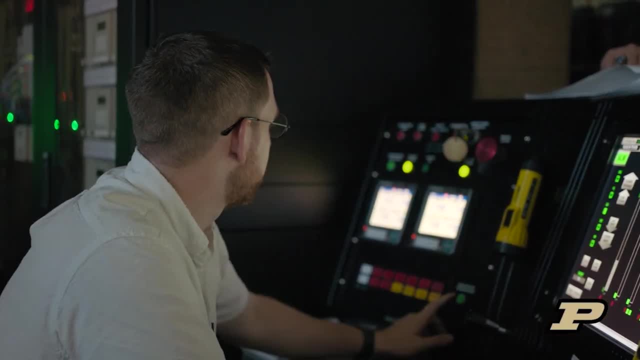 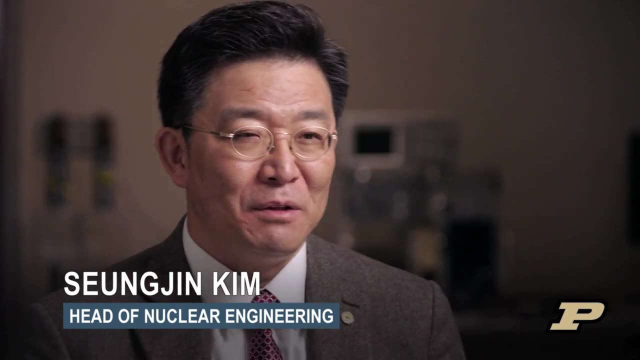 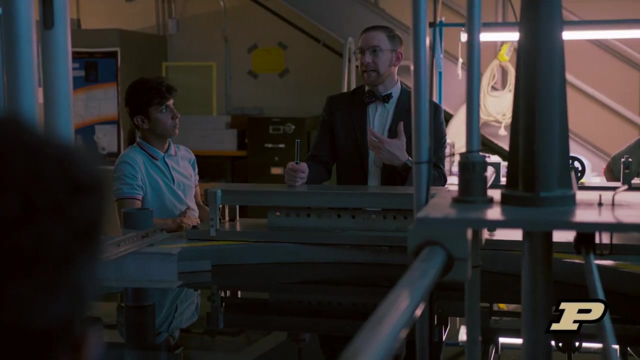 Delos Chilip, deejay. Director of helping niemand. human rights: make the difference between到 더욱 upstairs. 23 00 00 00 00. 00-00 00. actual departments, virtual labs & health workers. uger. cyber cutouts will lead to safer, more efficient atomic power in the future. If we had a very intelligent data analytics or artificially intelligent systems that could tell us "' Okay, in this scenario it may be best to choose to go this route — then of course human can make a judgment and decide. It can reduce, I think, significantly the error that human can make". Per 1, it seems, is the perfect сможsh cuts. 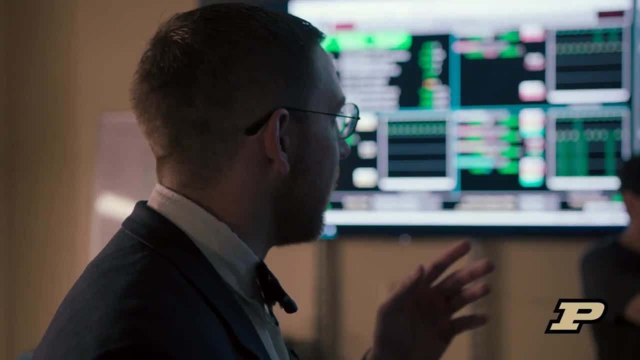 place to push nuclear power from its analog past into a digital future For Purdue University. I'm Miles O'Brien.